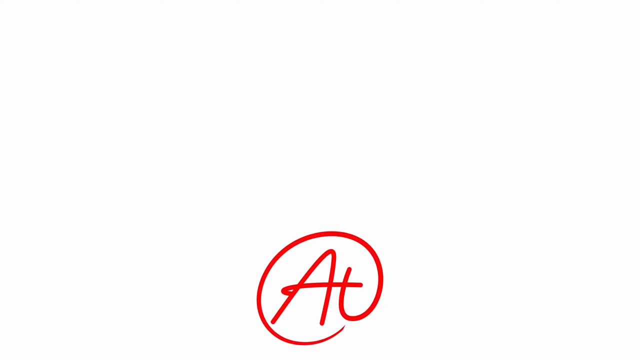 Hey guys, it's Mark from Ace Tutors and in this video I'm going to explain one of the most common probability distributions covered in STAT: the normal distribution. First I'll go over this concept at a high level. then I'll explain how this distribution is used to find probabilities. 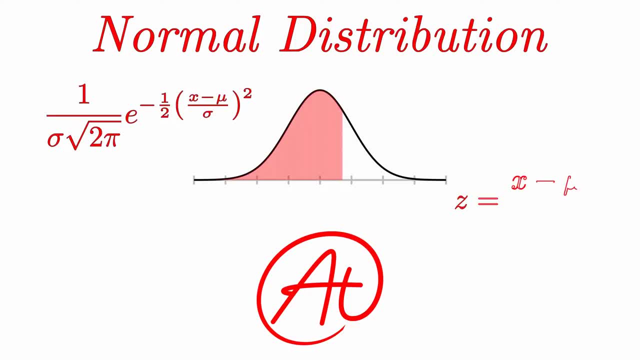 and finally, we'll finish things off with an example. And just quickly before I begin, if you would please consider tapping those subscribe and like buttons below to help us keep making videos like this for students like you. So now let's dive right in. First of all, a normal distribution looks like this: symmetric. 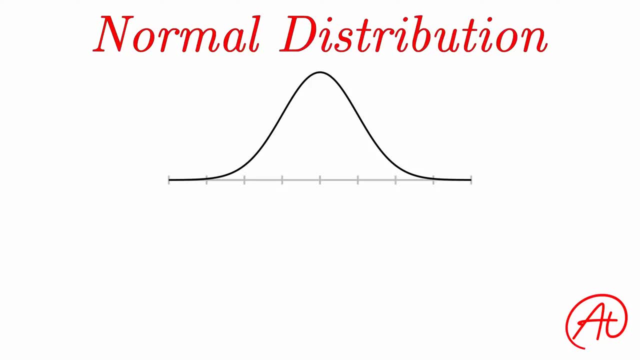 bell-looking thing, which is why it's often called a bell curve. Now, this curve is centered around the distribution's mean and spreads out with decreasing probability as you move away in either direction. Although the normal distribution technically continues indefinitely in either direction, it only really happens when you move away from it. So if you move away from a normal 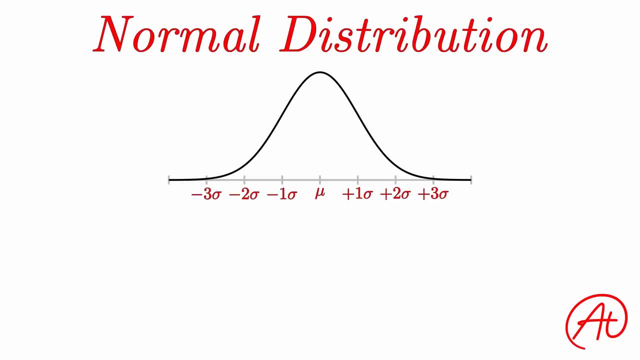 distribution. it only really happens when you move away from it. So if you move away from it, you'll notice that the normal distribution typically has significant probability values between 3 standard deviations below and above the mean. In fact, as a general rule of thumb, 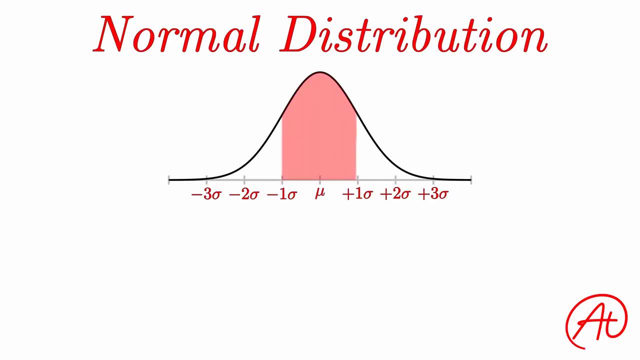 for a normal distribution: between plus or minus 1 standard deviation, there is 68% of the distribution's data. Between plus or minus 2 standard deviations, there is 95% of the data. Finally, between plus or minus 3 standard deviations, there is 99.7% of the data. 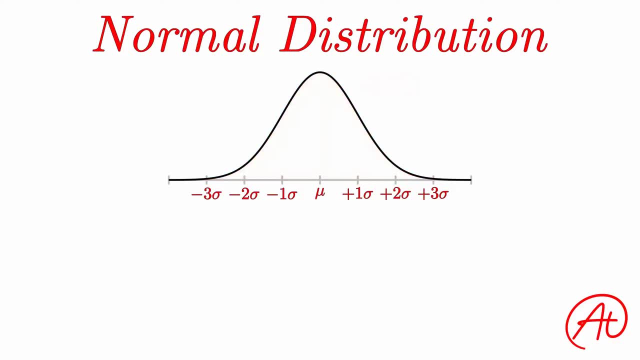 Now, the reason I called this distribution one of the most popular ones is because it can be used for so many types of real-world applications. For example, certain things like people's heights, weights and even IQ follow a normal distribution pretty closely. 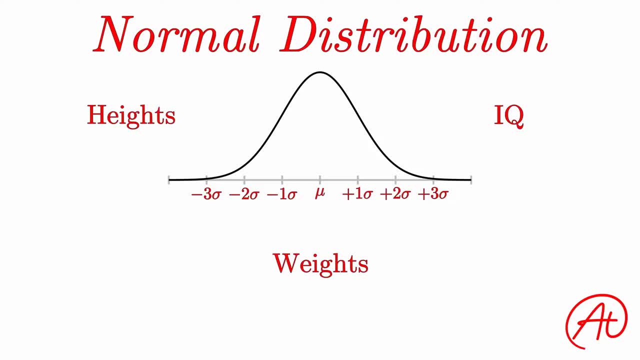 However, because the normal distribution is so widely applicable and each application comes with its own mean, standard deviation and, most importantly, units, this causes some problems. To solve this issue, instead of keeping the data in its original units, we get rid of. 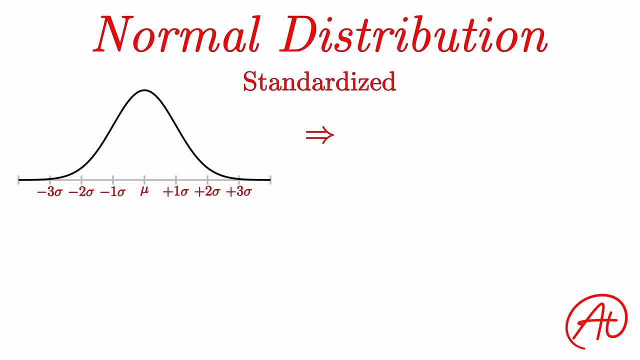 the units by doing what's called standardizing the data. Essentially, we take our original distribution and transfer it to have a mean of 0 and standard deviation of 1.. As a result, any normal distribution of any magnitude or unit type can be converted to. distribution. it only really happens when you move away from it. So, if you move away from it, it only really happens when you move away from it. So, if you move away from it, it only really happens when you move away from it. So if you move away from it. 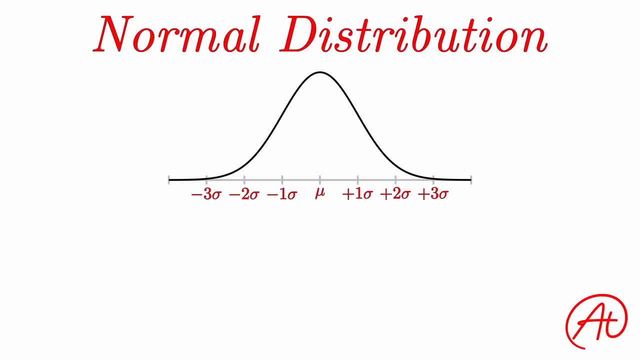 you might have significant probability values between three standard deviations below the mean. In fact, as a general rule of thumb for a normal distribution, between ±1 standard deviation, there is 68% of the distribution's data. Between ±2 standard deviations, there is 95% of the data. And finally between 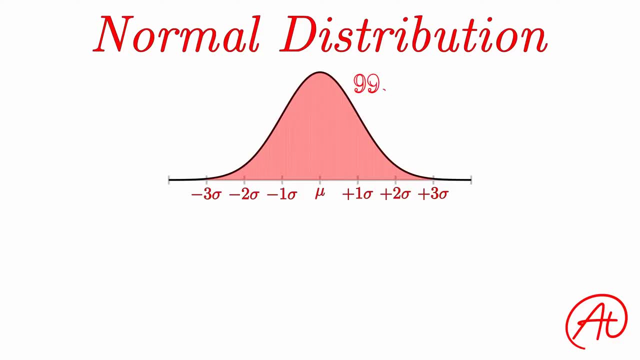 ±3 standard deviations, there is 99.7% of the data. Now, the reason I called this distribution one of the most popular ones is because it can be used for so many types of real-world applications, For example, certain things like people's heights, weights and even IQ. 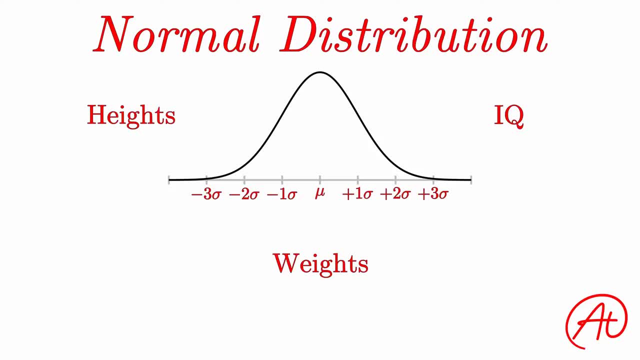 follow a normal distribution pretty closely. However, because the normal distribution is so widely applicable and each application comes with its own means, standard deviation and, most importantly, units, this causes some problems. To solve this issue, instead of keeping the data in its original units, 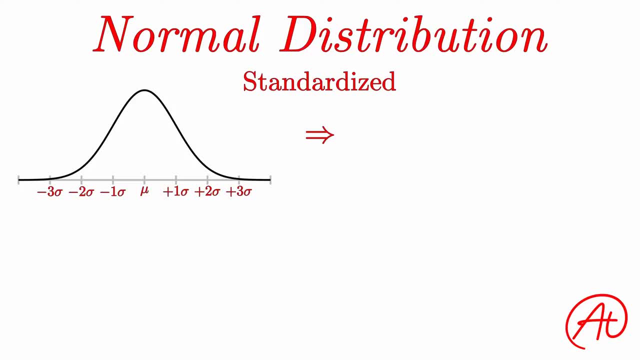 we get rid of the units by doing what's called standardizing the data. Essentially, we take our original distribution and transfer it to have a mean of 0 and standard deviation of 1.. As a result, any normal distribution of any magnitude or unit type. 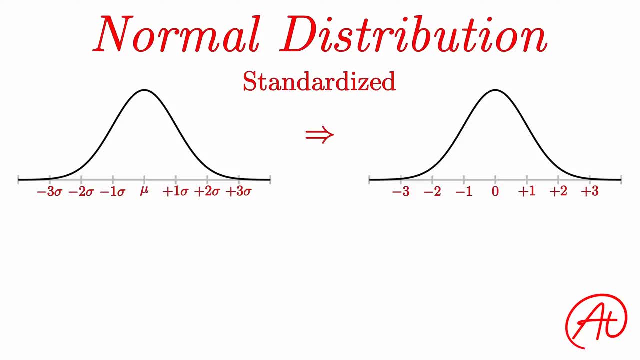 can be converted to be centered around 0 and extend more or less from negative 3 to positive 3.. Thank you for watching. Okay, that's cool, but how do we actually do that? Well, in order to standardize the data. 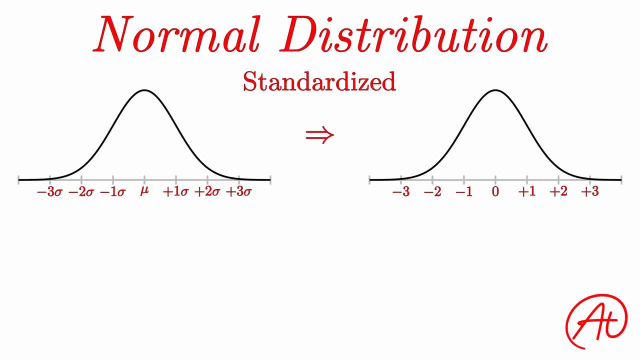 we need something you may have already heard about in your class, the infamous z-score, which has a formula: of z equals the data point x minus the mean mu divided by the standard deviation sigma. Essentially, what the z-score tells you is how many standard deviations a certain data point is away from the mean. 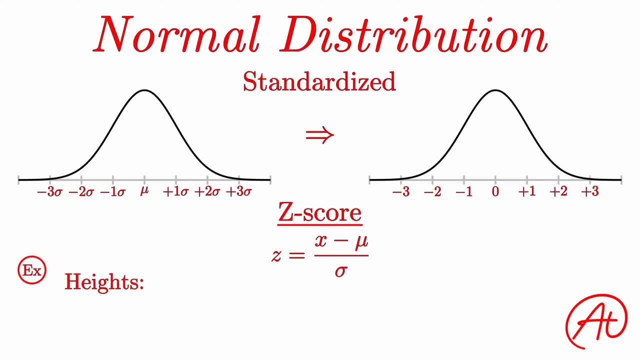 So, for example, if the heights of people in your stat class were normally distributed with a mean of 66 inches and standard deviation of 2 inches, your unstandardized distribution would look like this, centered at 66 inches and spreading out by increments of the standard deviation, like this: 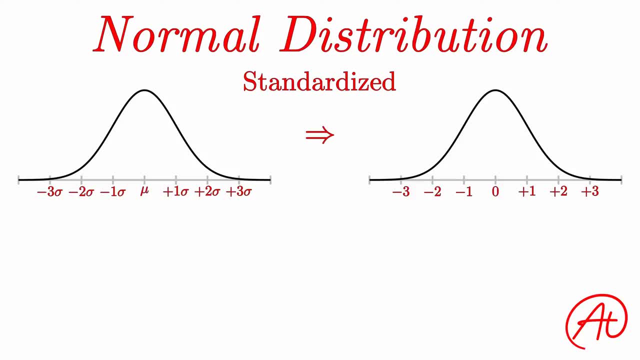 be centered around 0 and extend more or less from negative 3 to positive 3.. Okay, that's cool, but how do we actually do that? Well, in order to standardize the data, we need something you may have already heard. 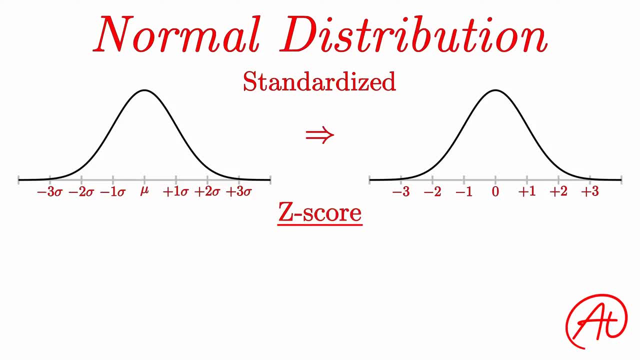 about in your class, the infamous z-score, which has a formula: of z equals the data point x minus the mean mu divided by the standard deviation sigma. Essentially, what the z-score tells you is how many standard deviations a certain data point is away from the mean. 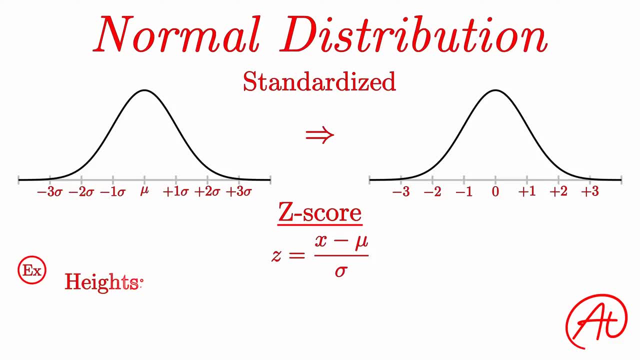 So, for example, if you want to know how many standard deviations a certain data point is away from the mean. So, for example, if you want to know how many standard deviations a certain data point is away from the mean. So, for example, if the heights of people in your stat class were normally distributed. 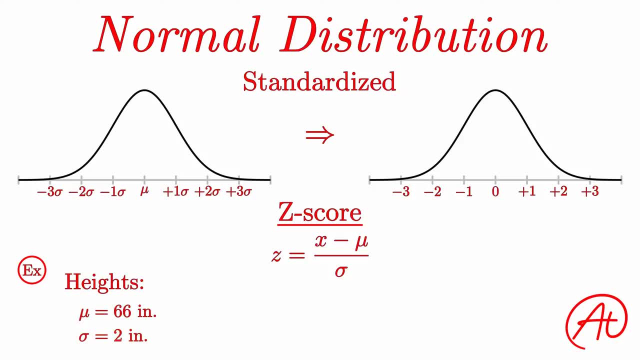 with a mean of 66 inches and standard deviation of 2 inches, your unstandardized distribution would look like this, centered at 66 inches and spreading out by increments of the standard deviation. like this, If you happen to have a height of 67 inches, you would fall right here in the distribution. 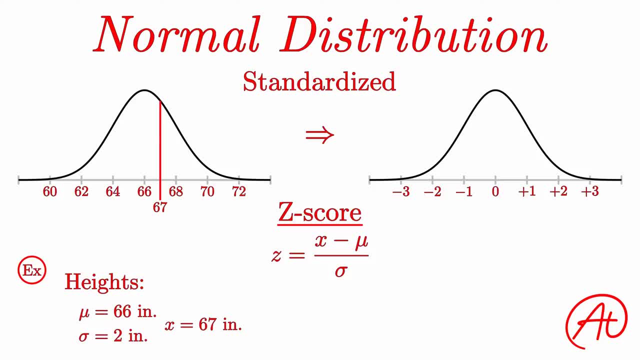 slightly above the mean. If we were to standardize your data point, we would find that the standard deviation of your z-score equals 67 minus 66 divided by 2, which is 1 over 2, or 0.5.. 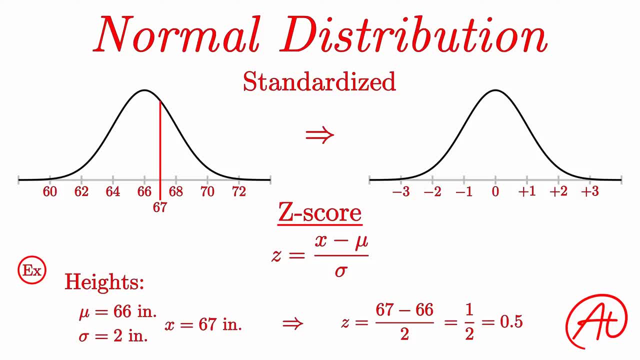 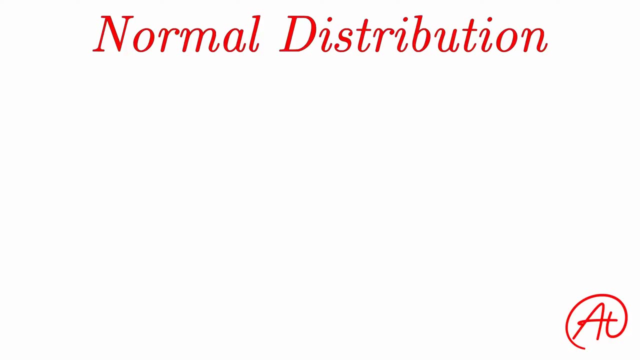 This z-score of 0.5 means that your data point is half of a standard deviation above the mean and located here, the same exact location in the distribution as before. Alright, now that we covered how and why we standardize normal distributions, let's move. 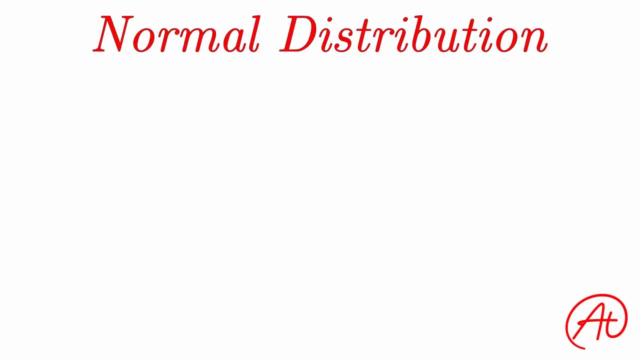 on to the most important part of all: probabilities. Now, unlike the other distributions we covered, there isn't a nice and pretty formula for figuring out probabilities for the normal distribution. Instead, to calculate probabilities for this distribution, we have to rely on using charts. 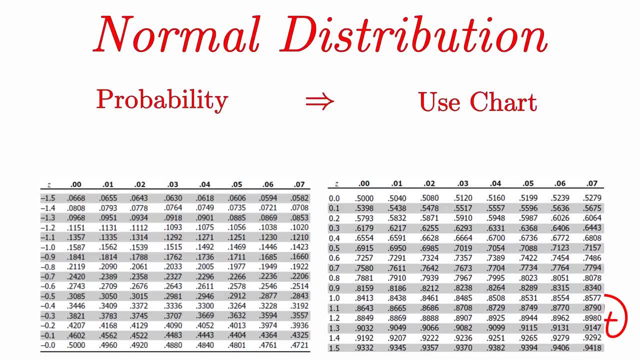 which might look like these, where numbers on the leftmost column and topmost row correspond to your z-score and the interior numbers correspond to those z-scores associated with the associated probability values. So, for example, if your z-score was 0.63, you'd go down to the 0.6 row corresponding. 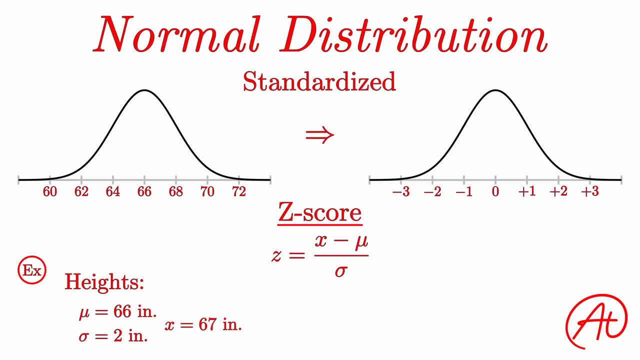 If you happen to have a height of 67 inches, you would fall right here in the distribution, slightly above the mean. If we were to standardize your data point, we would find that your z-score is 0, and your z-score equals 67 minus 66 divided by 2,. 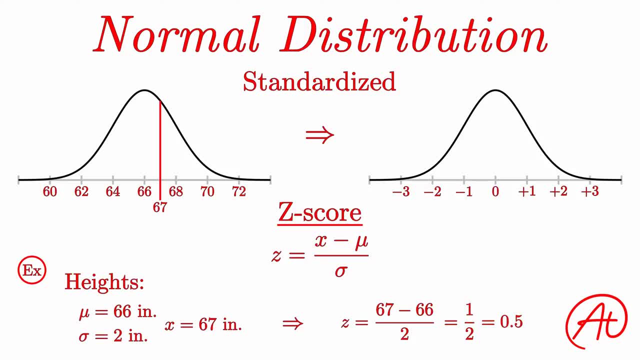 which is 1 over 2, or 0.5.. This z-score of 0.5 means that your data point is half of a standard deviation above the mean and located here the same exact location in the distribution as before. 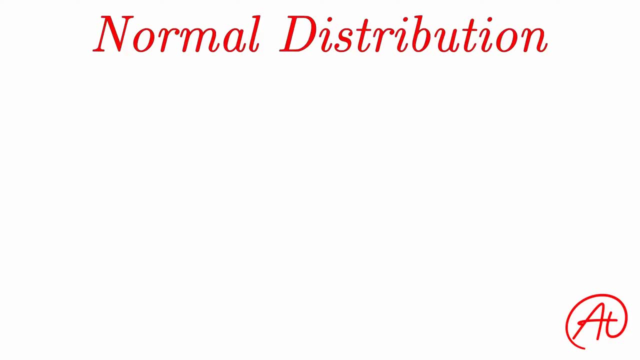 All right, now that we've covered how and why we standardize normal distributions, let's move on to the most important part of all: probability distributions, and that's well, probability. Now, unlike the other distributions we covered, there isn't a nice and pretty formula for figuring out probabilities for the normal distribution. 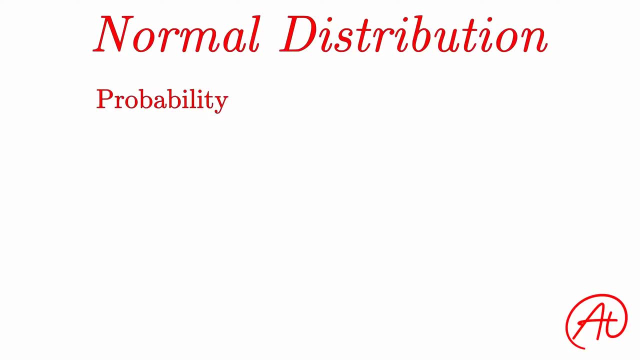 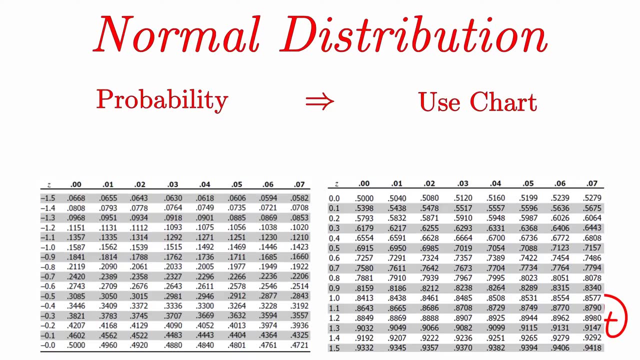 Instead, to calculate probabilities for this distribution, we have to rely on using charts which might look like these, where numbers on the leftmost column and topmost row correspond to your z-score and the interior numbers correspond to those z-scores associated probability. 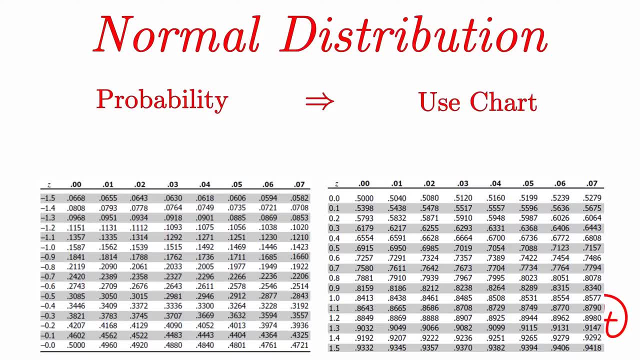 So, for example, if your z-score was 0.63, you'd go down to the 0.6 row, corresponding to the 6 in the z-score's tenths place, and over to the 0.03 column. 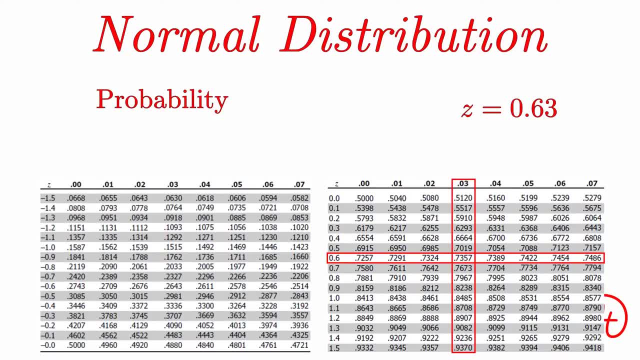 corresponding to the 3 in the z-score's hundredths place to get the associated probability value of 0.7357.. Okay, but what does that value actually mean? Well, in order to know that, it's very important to know that the probability value of 0.7357 is 0.7357.. 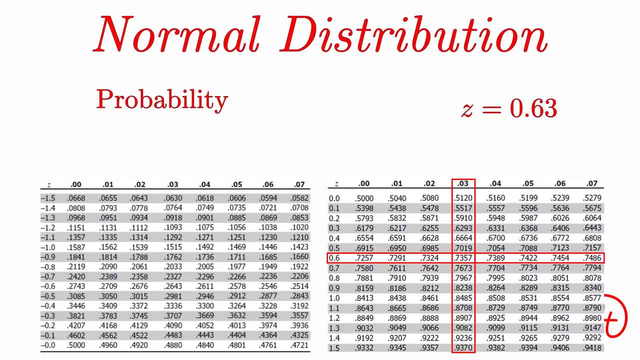 It's also important to understand what values the z-chart you're looking at gives you. For these z-charts, it happens to give you the area or probability of being to the left of your z-score. So, for our previous example, based on the value found in the chart, 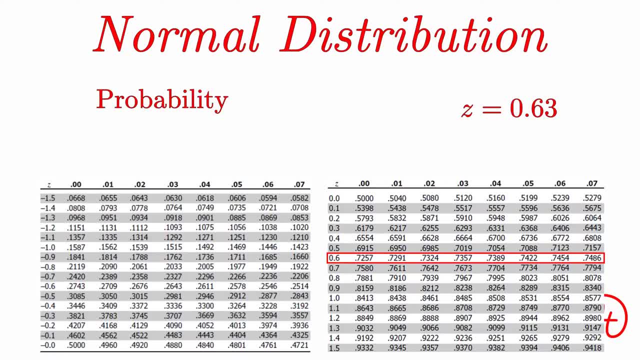 to the 6 in the z-score's tenths place and over to the 0.03 column corresponding to the 3 in the z-score's hundredths place, to get the associated probability value of 0.7357.. Okay, but what does that value actually mean? 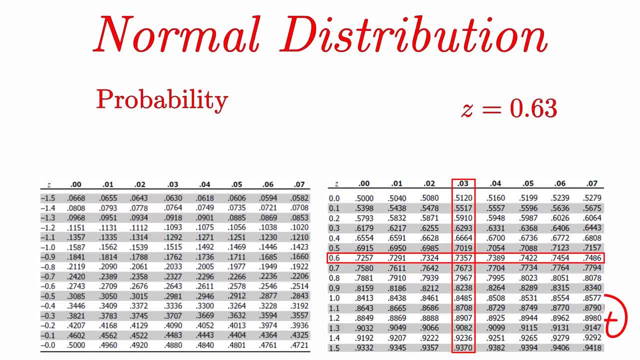 Well, in order to know that, we need to know the value of the z-score. It's very important to understand what values the z-chart you're looking at gives you. For these z-charts, it happens to give you the area or probability of being to the left. 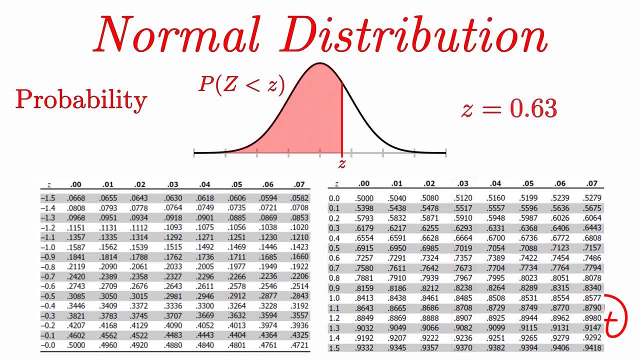 of your z-score. So for our previous example, based on the value found in the chart, there is a 73.57% chance of having a z-score less than 0.63.. And one last quick note: it's also important to make sure you are using the correct chart. 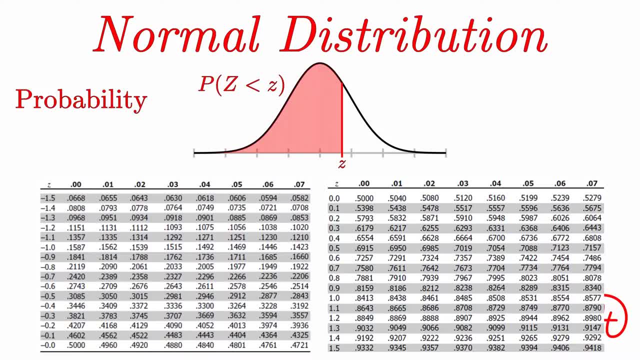 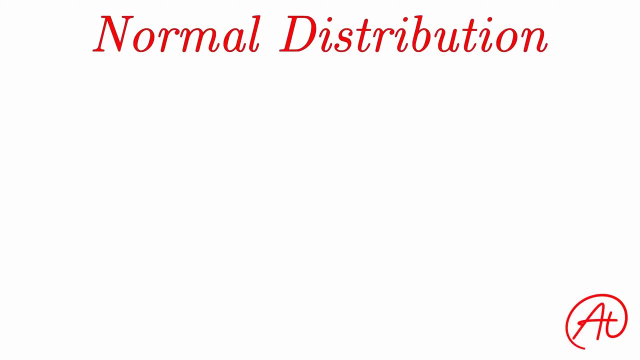 based on whether you have a negative or positive z-score. The one on the left is for negative z-scores, or values below the mean, and the one on the right is for positive z-scores, or values above the mean. Alright, I know I've been throwing a ton of info at you, so let's solidify all of this. 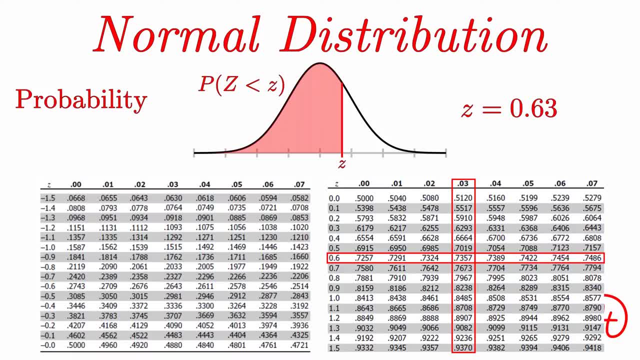 there's a 73.57% chance of having a z-score less than 0.63.. And one last quick note: it's also important to make sure you are using the correct chart, based on whether you have a negative or positive score. 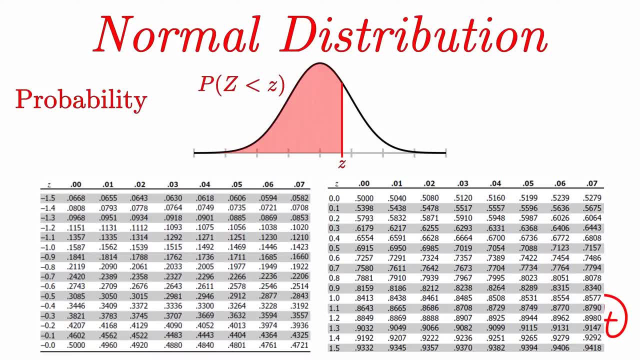 The one on the left is for negative z-scores, or values below the mean, and the one on the right is for positive z-scores, or values above the mean. Alright, I know I've been throwing a ton of info at you. 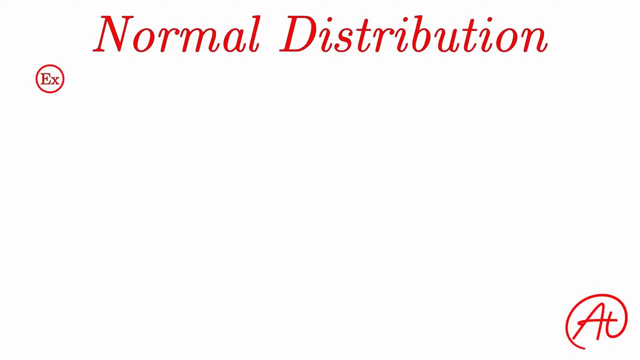 so let's solidify all of this with a quick example. So you love pizza, but your local pizza shop's pizzas have been looking smaller and smaller lately. They claim that their large is at least 16 inches or it's free. 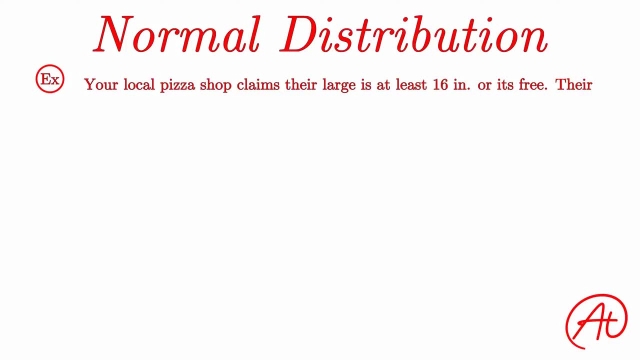 Over your expansive pizza area, you've found that their pizzas are normally distributed in size, with a mean of 16.3 inches and standard deviation of 0.2 inches. Now you want to know what the probability is of getting a free pizza. 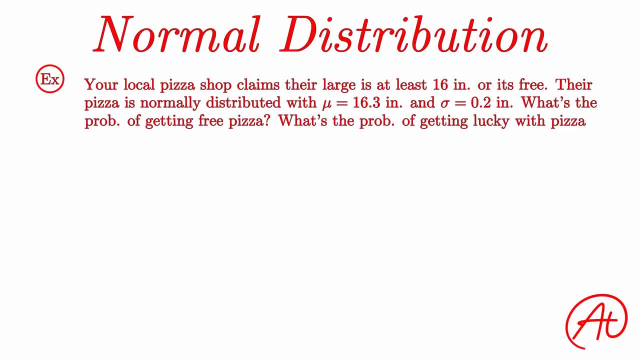 Also, what's the probability of getting lucky with a pizza that's over 16.5 inches? And just because you love stat and love eating pizza, what's the probability of getting a pizza that's between 15.95 inches and 16.6 inches? 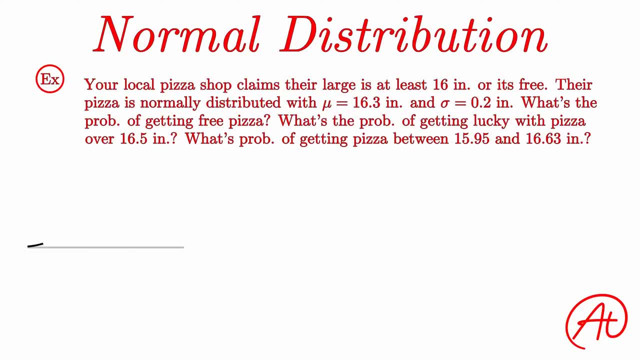 Okay, first, let's draw our normal distribution centered at the mean of 16.3 inches, And we want to find the probability of getting a pizza that is less than 16 inches, which looks like this. Now our first step for these problems. 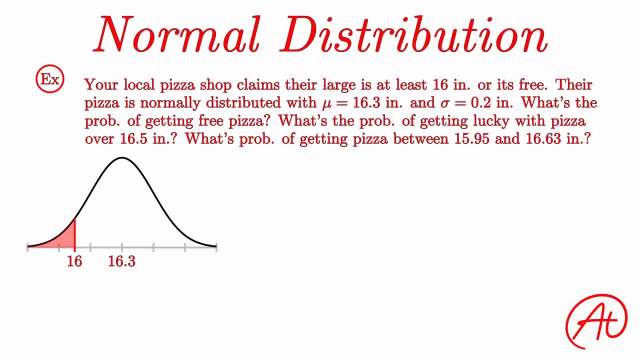 is always going to be. standardize our distribution Using our z-score equation and plugging in our data point of 16,, we get 16 minus 16.3 divided by 3. Which gives us a z-score of 0.2,. 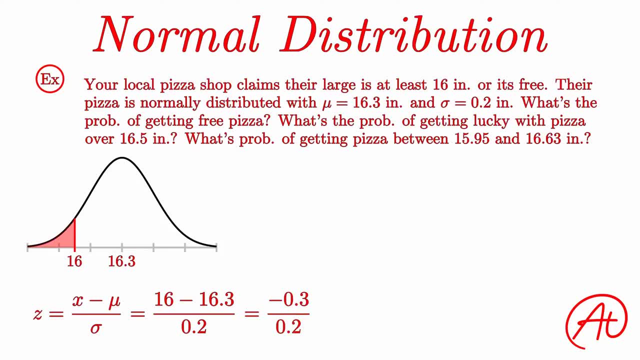 or negative 0.3 over 0.2, which gives us a z-score of negative 1.5.. So, instead of finding the probability of a pizza x being less than 16 inches, we are now finding the probability of a pizza having a z-score less than negative 1.5.. 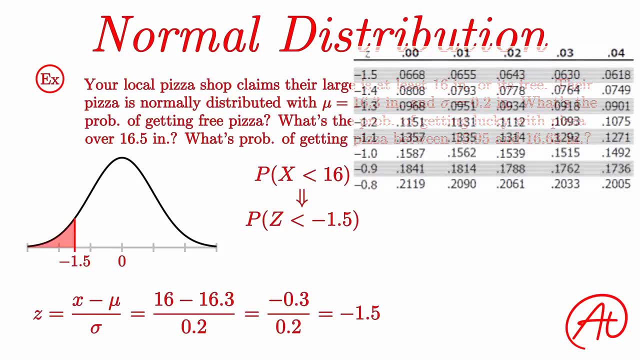 Now that we have a z-score, we can use our z-chart to find its associated probability. Looking at row negative 1.5, and column 0.00,, we find a probability of 0.0668.. Since we want to find the probability of being less than our z-score, 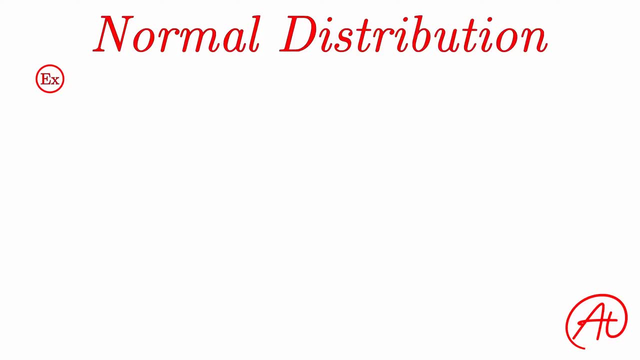 with a quick example. So you love pizza, but your local pizza shop's pizzas have been looking smaller and smaller lately. They claim that their large is at least 16 inches or it's free. So you love pizza, but your local pizza shop's pizzas have been looking smaller and smaller lately. 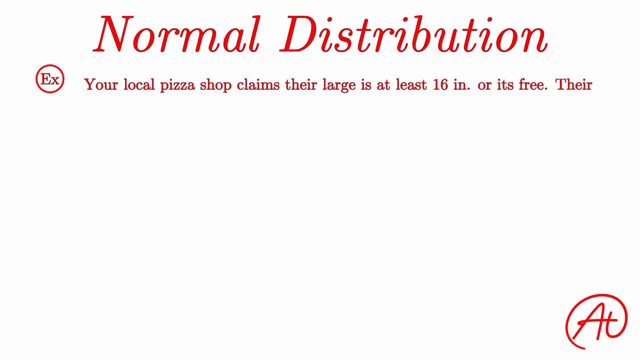 Over your expansive pizza-eating career, you've found that their pizzas are normally distributed in size with a mean of 16.3 inches and standard deviation of 0.2 inches. Now you want to know what the probability is of getting a free pizza. 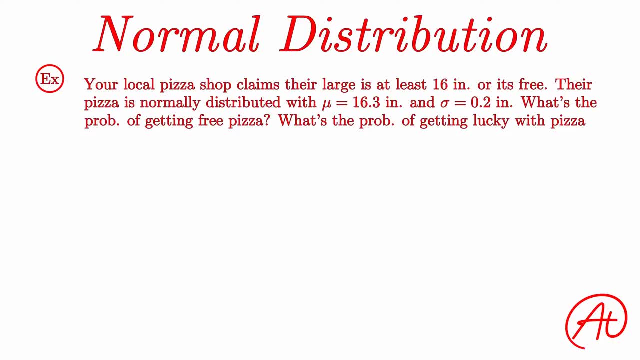 Also, what's the probability of getting lucky with a pizza that's over 16.5 inches? And just because you love stat and love eating pizza, what's the probability of getting a pizza between 15.95 and 28.10 inches? 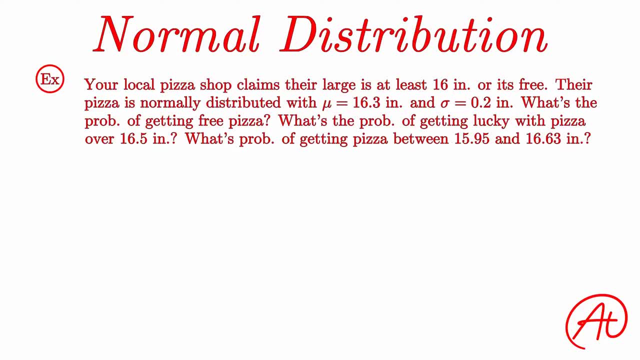 inches and 16.63 inches. Okay, first let's draw our normal distribution centered at the mean of 16.3 inches, and we want to find the probability of getting a pizza that is less than 16 inches, which looks like this. Now our first step for these. 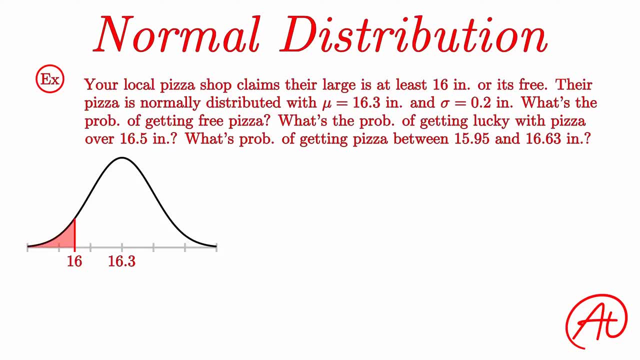 problems is always going to be: standardize our distribution. Using our z-score equation and plugging in our data point of 16,, we get 16 minus 16.3 divided by 0.2, or negative 0.3 over 0.2, which gives us a z-score of negative 1.5.. 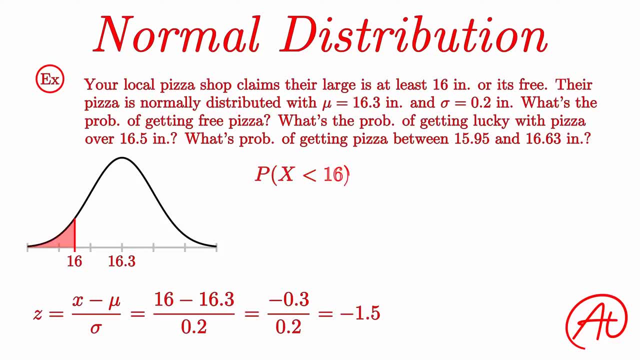 So, instead of finding the probability of a pizza X being less than 16 inches, we are now finding the probability of a pizza having a z-score less than negative 1.5.. Now that we have a z-score, we're going to find the probability of a pizza having a z-score less than negative 1.5.. Now that we have a z-score, 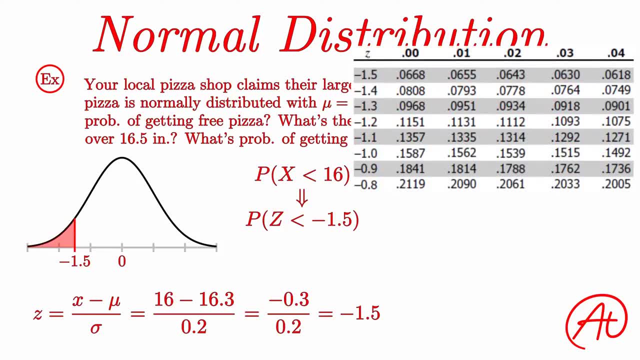 we can use our z-chart to find its associated probability. Looking at row negative 1.5 and column 0.00, we find a probability of 0.0668.. Since we want to find the probability of being less than our z-score, and that being 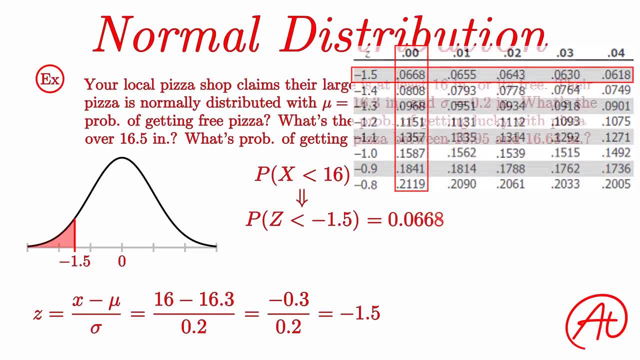 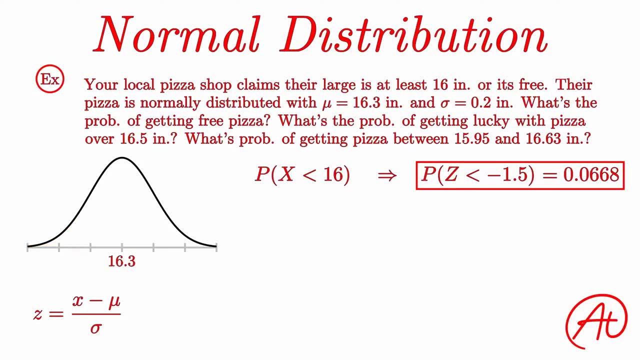 exactly what the chart gives us. we're done. We have a 6.68% chance of getting a free pizza. Next, we want to find the probability of a pizza being over 16.5 inches, Like before. our first step is to find this. 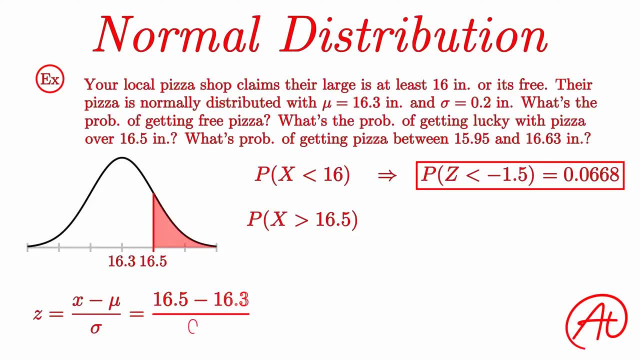 data point z-score, which equals 16.5 minus 16.3 divided by 0.2, or 0.2 over 0.2 or just 1.. So this time we want to find the probability of having a z-score. 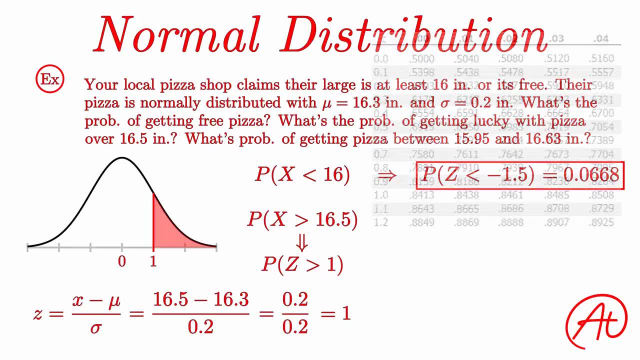 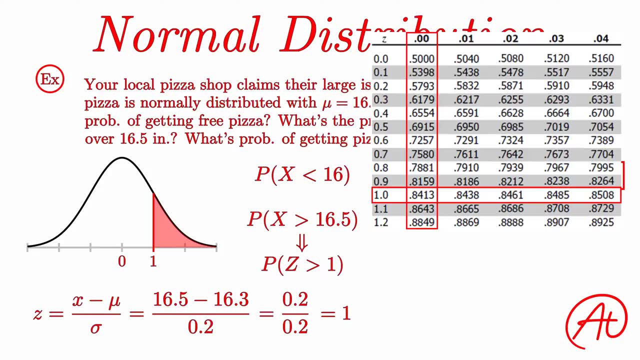 higher than 1.. Looking at our chart, for our z-score, we go to row 1.0 and column 0.00 and column 0.00.. to get a probability of 0.8413.. But keep in mind, this chart always gives you the probability to the left of your. 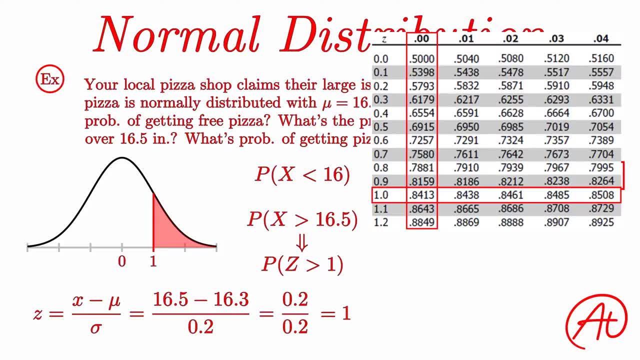 z-score. Since the area under the entire distribution is always equal to 1 and the area to the left is 0.8413,, we can get the area to the right by subtracting 1-0.8413 to get our final answer of 0.1587. 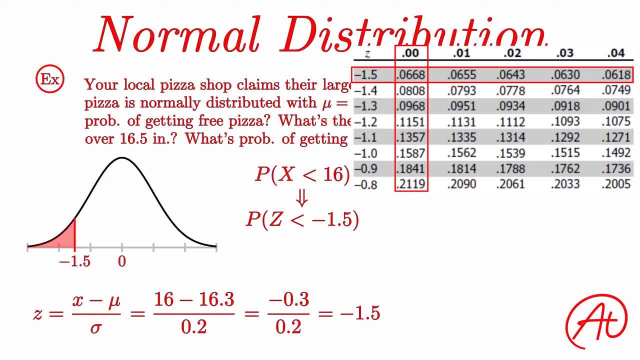 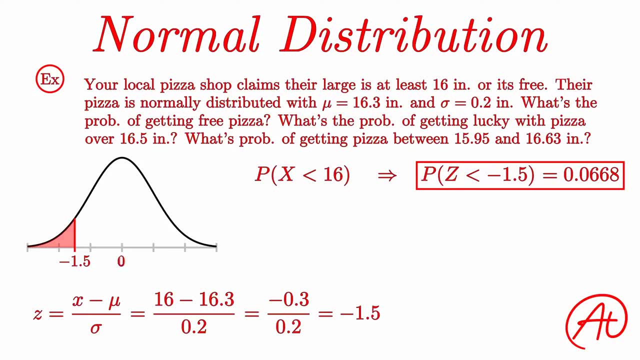 and that being exactly what the chart gives us, we're done. We have a 6.68% chance of getting a free pizza. Next, we want to find the probability of a pizza being over 16.5 inches, Like before. 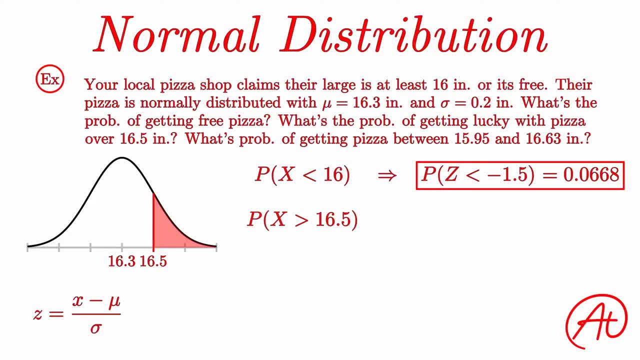 our first step is to find this data point's z-score, which equals 16.5 minus 16.3 divided by 0.2, or 0.2 over 0.2, or just 1.. So this time, 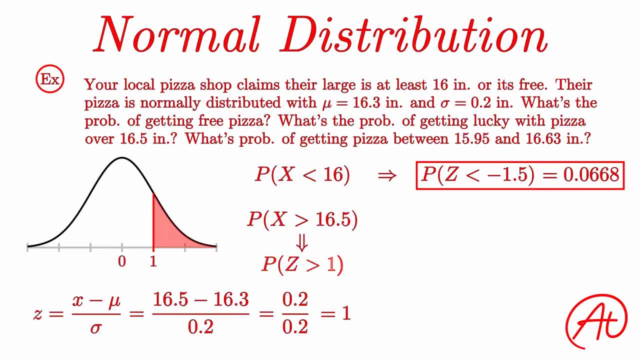 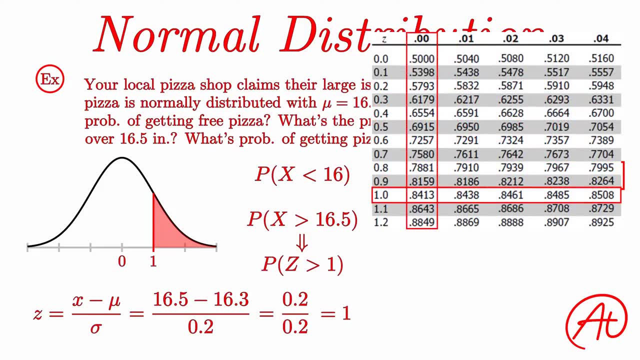 we want to find the probability of having a z-score higher than 1.. Looking at our chart for our z-score, we go to row 1.0 and column 0.00 to get a probability of 0.8413.. But keep in mind: 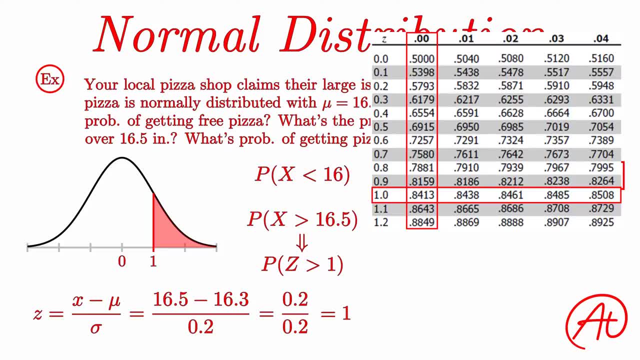 this chart always gives you the probability to the left of your z-score. Since the area under the entire distribution is always equal to 1, and the area to the left is 0.8413,, we can get the area to the right by subtracting 1 minus 0.8413. 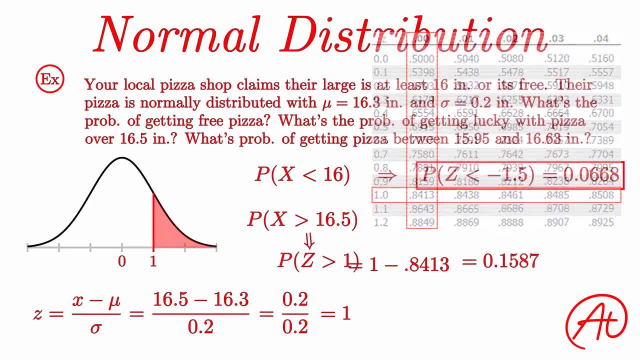 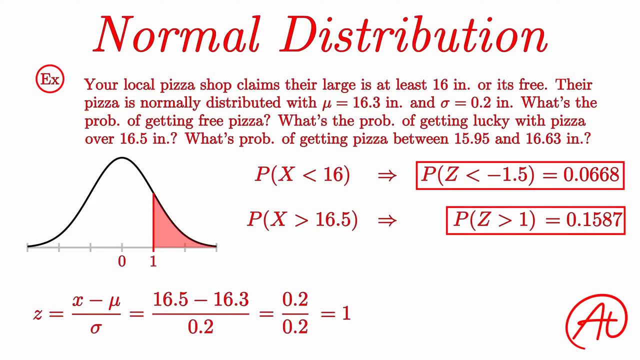 to get our final answer of 0.1587, or a 15.87% chance of getting a pizza larger than 16.5 inches- Not too shabby. Finally, we want to find the probability of getting a pizza between 15.95 and 16.63 inches. 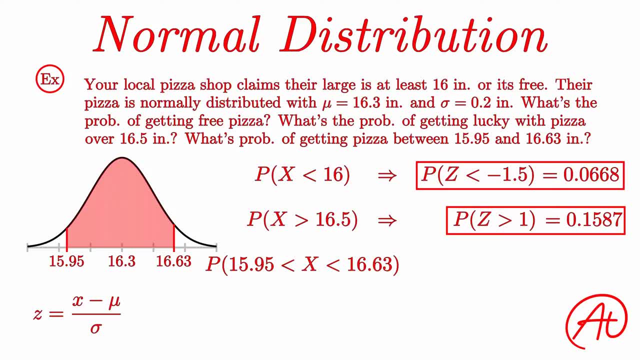 First, as always, let's find some z-scores. For 15.95, we get negative 0.35 divided by 0.2, or negative 1.75.. And for 16.63, we get 0.33 divided by 0.2,. 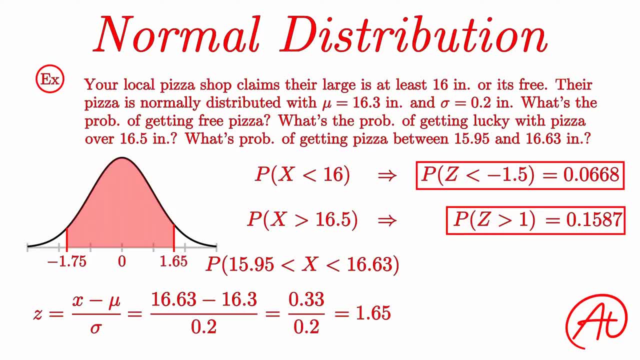 or 1.67.. So we get 1.65.. Alright, we have our z-scores now, but how do we use them to find the area between them? Well, one way to do it would be first looking the chart for the larger z-score. 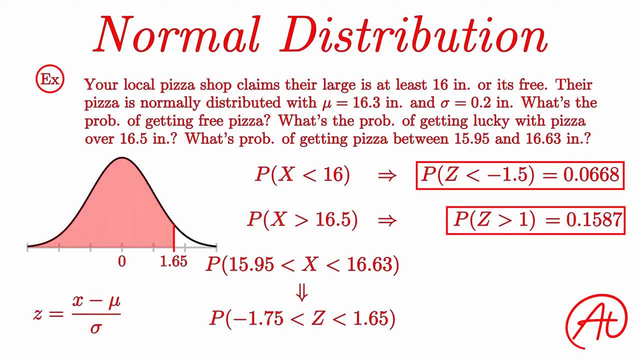 This would get you this area here to the left of 1.65.. Then you can find the area to the left of the smaller z-score, which would get you this area in the tail here. Once you have those, you can subtract the smaller area from the larger area. 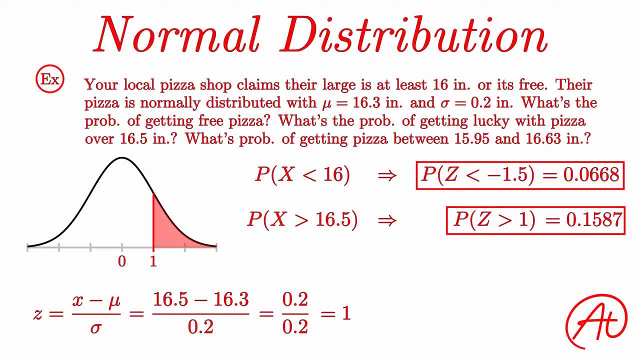 or a 15.87 percent chance of getting a pizza larger than 16.5 inches. Not too shabby. Finally, we want to find the probability of getting a pizza between 15.95 and 16.63 inches. First, as always, let's find some z-scores. 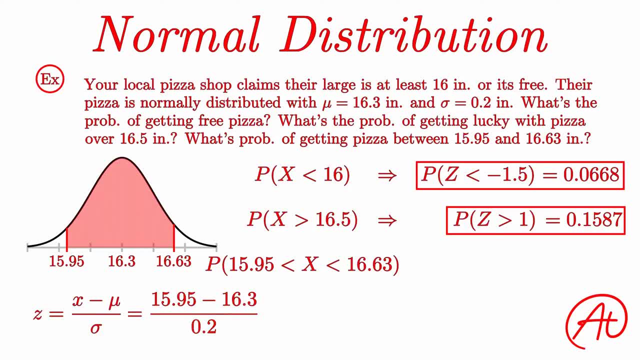 For 15.95, we get negative 0.35 divided by 0.2, or negative 1.75.. And for 16.63, we get 0.33 divided by 0.2 or 1.65.. 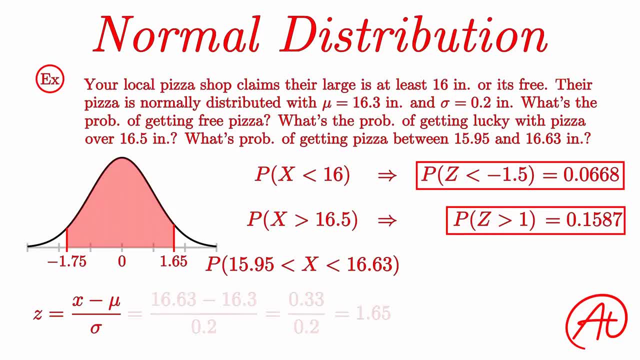 Alright, we have our z-scores now, but how do we use them to find the area between them? Well, one way to do it would be first look in the chart for the larger z-score. This would get you this area here to the left. 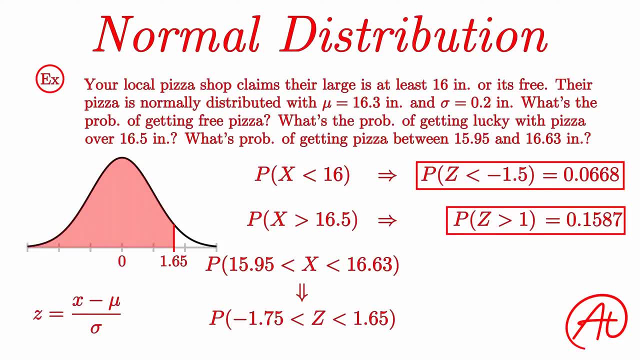 of 1.65.. Then you can find the area to the left of the smaller z-score, which would get you this area in the tail here. Once you have those, you can subtract the smaller area from the larger area to leave you with the area in between them. 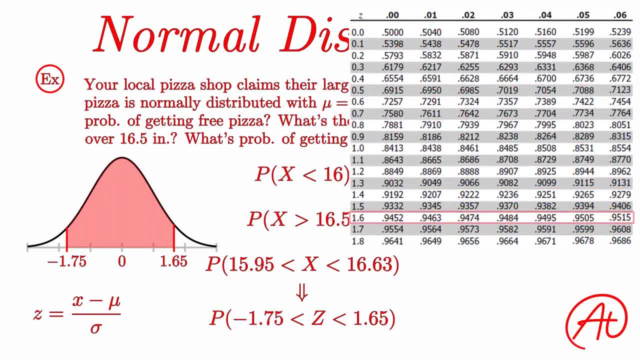 Looking in our positive z-score chart, we find the area below a z-score of 1.65 is 0.9505.. And then, looking in our negative z-score chart, we find the area below a z-score of negative 1.75. 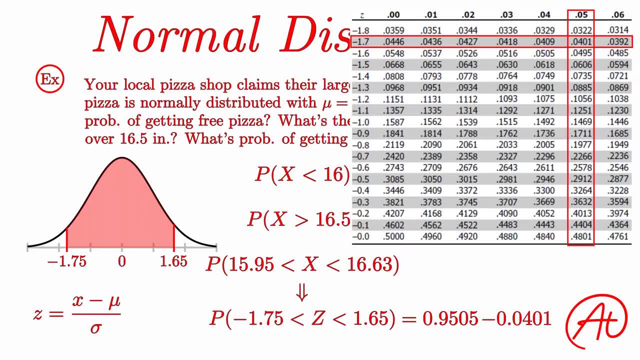 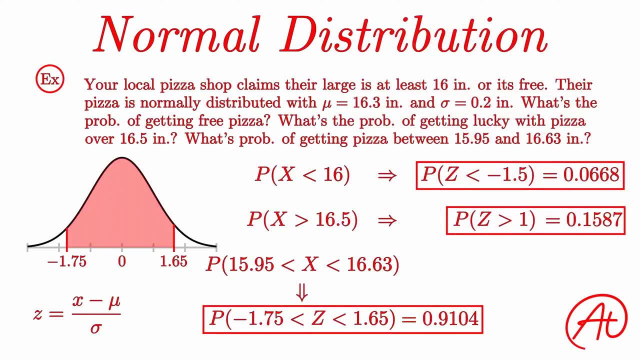 is 0.0401.. Subtracting these values, we get our answer of 0.9104, or a 91.04% chance of getting a pizza between 15.95 and 16.63 inches. So that right, there is the normal distribution. 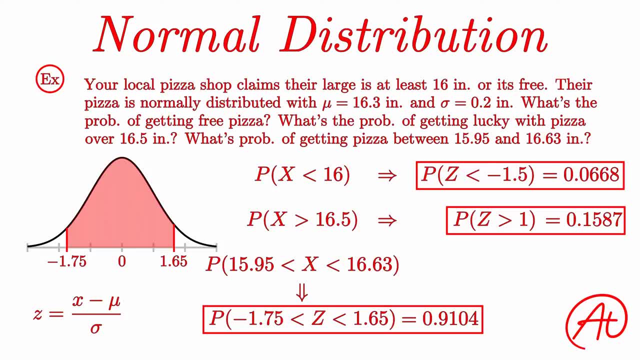 If you found this video helpful, please hit that subscribe button down below to support us making more videos for you. If you didn't, please leave us a comment down below to let us know what we can do better. Thanks again for watching and remember. you have big dreams. don't let a class get in the way.